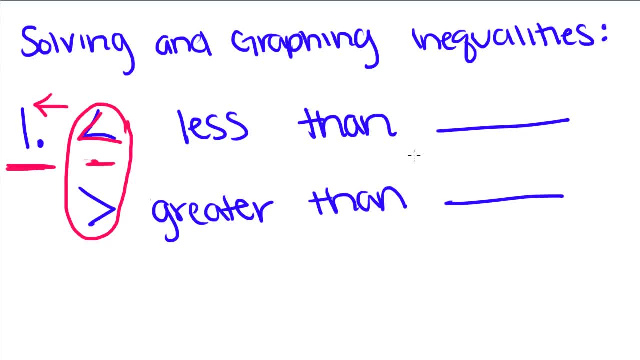 that this is less than or equal to this, than this, and that this is greater than this. So, now that we know that, I'm going to show you what a basic inequality looks like where s is greater than 6, and we always look at. 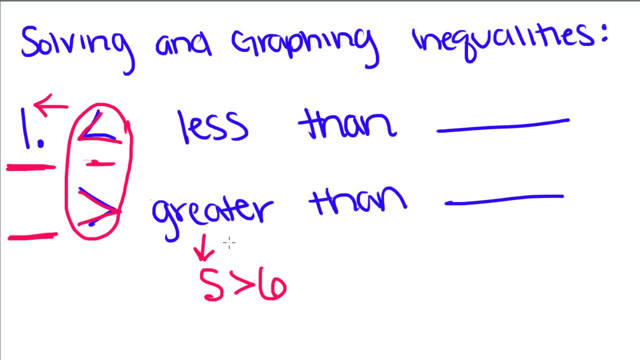 this inequality symbol from the variables perspective, because we could write this as this: which means that 6 is less than s, but it means that s is greater than 6.. So s is greater than 6, or we could say that t is less than 7, and those are what basic inequalities. 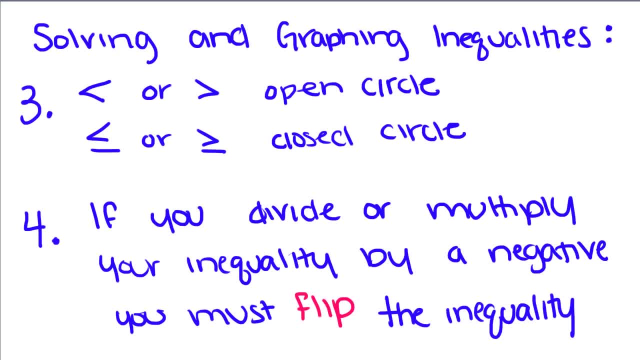 look like. So when we solve our inequalities, we're going to graph them, and you always graph the solution to an inequality. So when you have an inequality that has less than or equal- I'm sorry if you have an inequality. 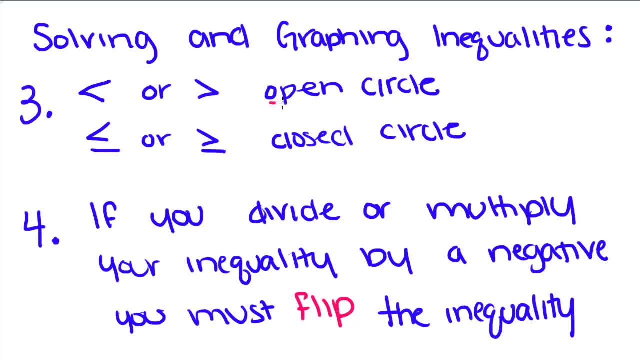 that's less than or greater than, when you graph it, you're going to use an open circle and that's not going to really make sense to you right now, but it will in a minute when we go until graphing. but if you have less than or equal to or greater than or, 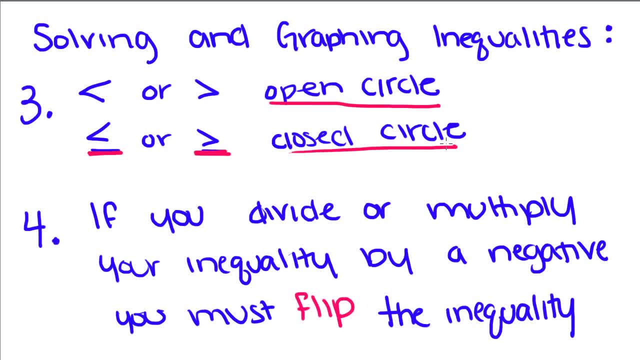 equal to 2, it's going to be a closed circle. And the most important thing to remember when solving inequalities is that if you divide or multiply your inequality by a negative, you must flip your inequality. So if I had negative, x is less than 2, when I divide by the negative, 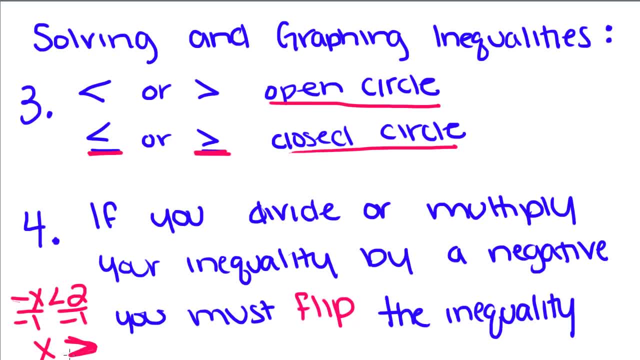 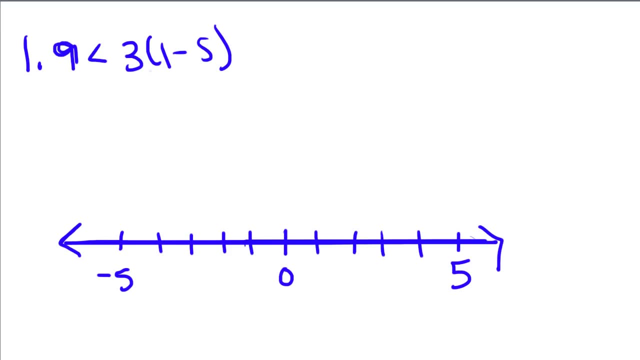 1, I'm going to get x- is greater than negative 2. That inequality sign has to flip, Otherwise you're going to get the wrong answer. So now let's do an example. 9 is less than 3 times the quantity of 1 minus s, And this is an s. if you couldn't tell, sorry, Kind of looks. 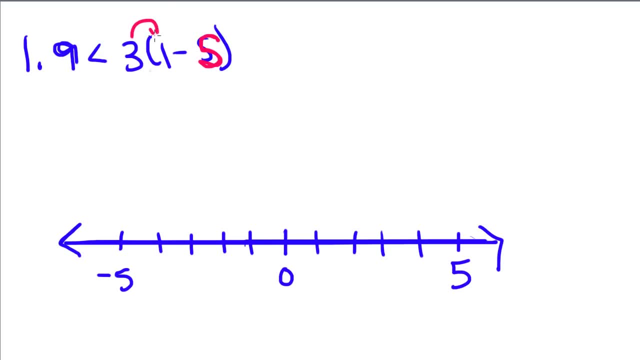 like a weird 5.. So first thing we're going to do is distribute that 3 over 9 is less than 3 minus 3s. I'm going to subtract 3 from both sides and I get 6 is less than negative 3s. I'm going to divide by negative 3 and negative 3.. And 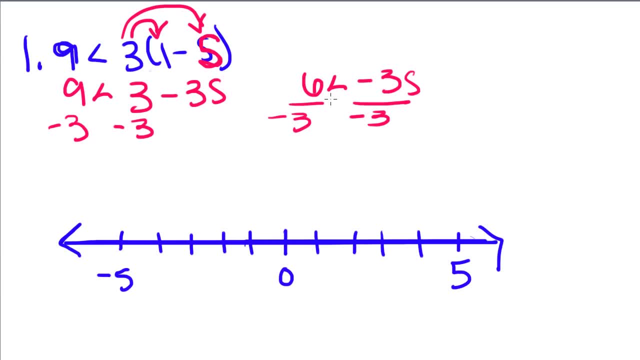 when you solve this. this is what you want to think. If you divide by a negative 3, you get a negative. If you divide by a negative, then you flip your sign. So negative 2, and we're going to flip it- is greater than s. So that means s is less than negative 2.. Either 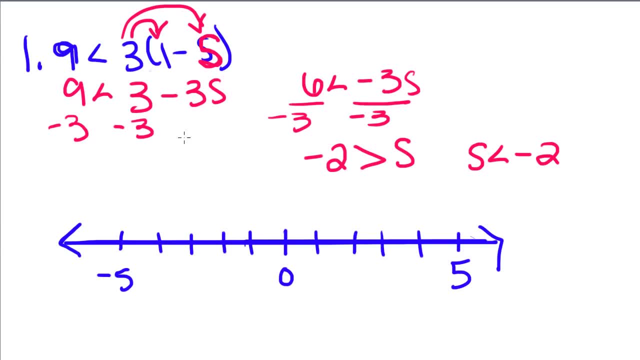 way is correct. So when I said, when we graph it on a number line, we're going to graph it on a number line that looks like this. So we're going, going, going, going, find negative 2 on the number line, which will be right here, and we're going to put 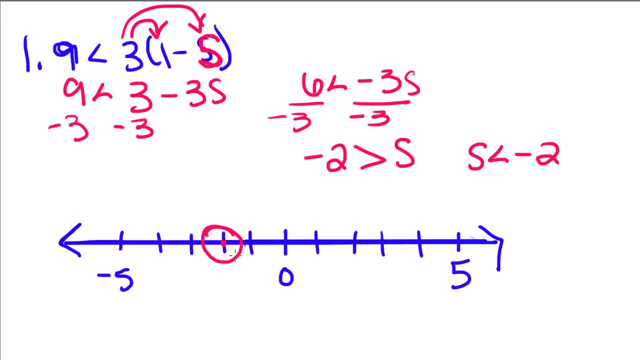 a circle over negative 2.. Now remember: if it's just less than or greater than, it's going to have an open circle, and if it's less than or equal to, or greater than or equal to, we're going to have a closed circle. So, since it's only less than, we're going to 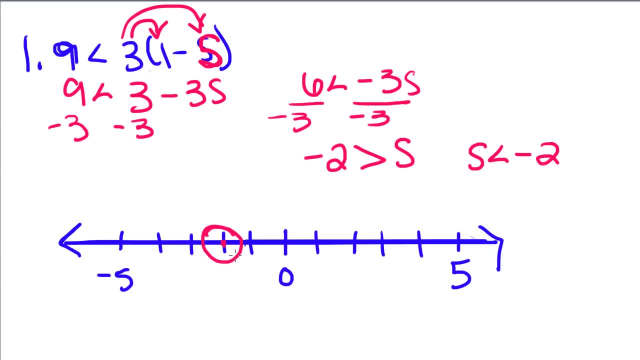 have an open circle and we're going to shade the direction of the inequality. So there's two ways you can remember this. You can remember that this inequality points to the left, so I'm going to shade To the left. or you can think of it more mathematically and we're going to put an arrow right here. 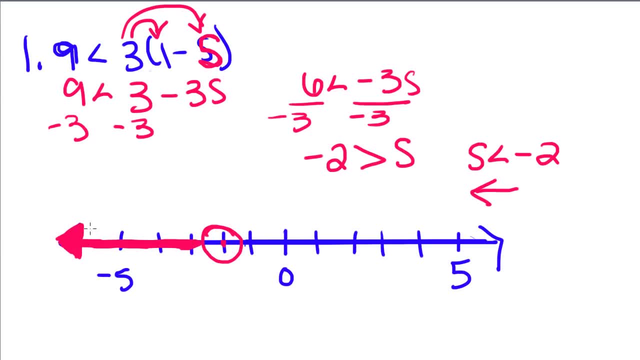 because, remember, lines go on forever. or you could plug in a number that's on the left of your circle, which would be like negative 4.. Well, is negative 4 less than negative 2?? Yes, because, remember, as we go, as we get more numbers, we're going to have a circle. 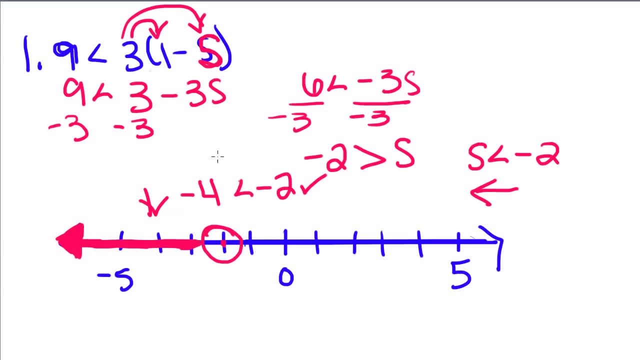 over negative. we're decreasing in value. And then you would pick a number to your right to make sure that it doesn't work to your right. Well, is 2 less than negative 2?? No, it's greater than negative 2, so that's how you know that you were supposed to shade. 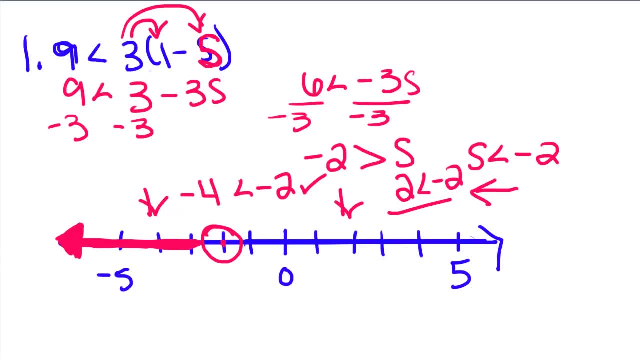 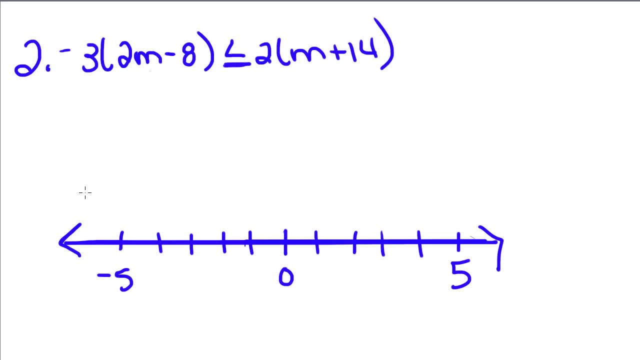 it this way. So we have one more example that we're going to do So negative 3 times the quantity of 2m minus 8 is less than or equal to 2 times the quantity of m plus 2.. So first, 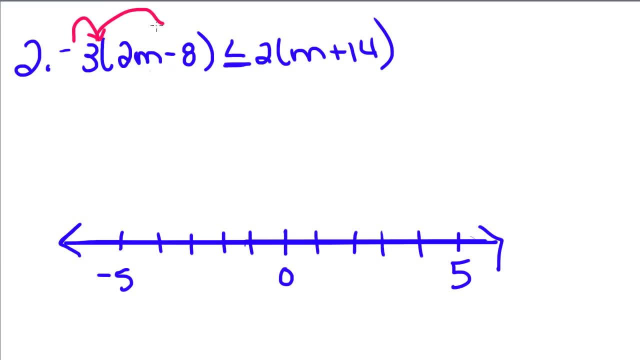 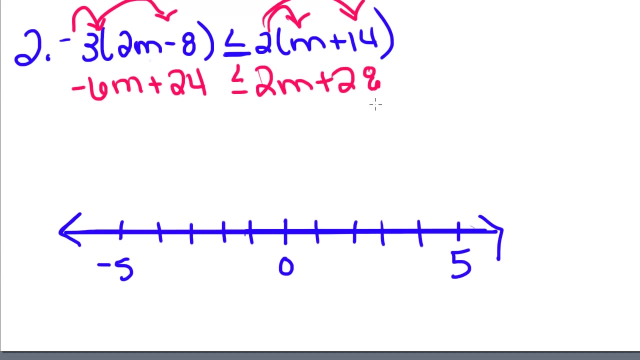 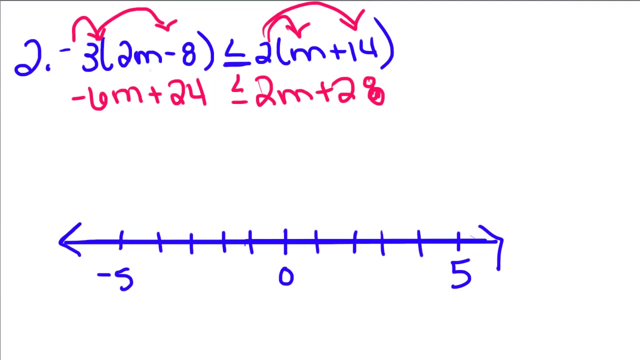 thing we're going to do is distribute on both sides of the equation, So we have negative 6m plus 24, less than or equal to, 2m plus 28.. Now some of you might say that well, didn't we multiply by a negative? Yes, we did, but we don't flip the sign yet, because we only 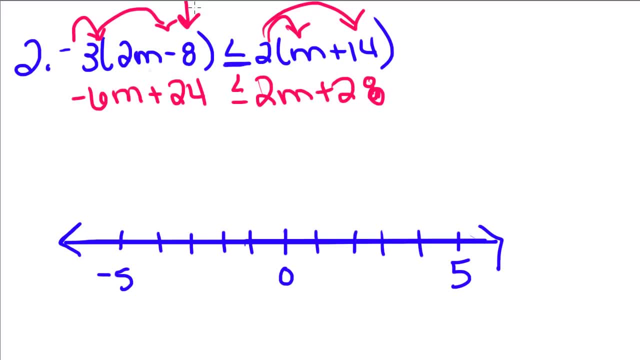 multiplied one side by a negative. It only affects your inequality when you have to multiply both sides or divide both sides by a negative. So then I'm going to move the 2m this way and this is going to be: I'm going to subtract 2m from both sides so this becomes negative: 8m plus 24 less than. 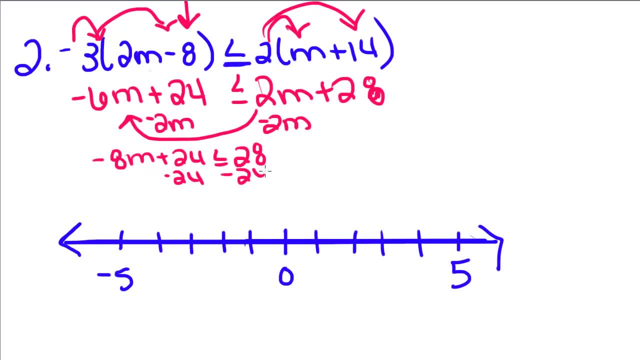 or equal to 28.. I'm going to subtract 24 from both sides and I get negative 8m is less than or equal to 4.. So I'm going to divide by negative 8 and divide by negative 8.. So, since I divided,